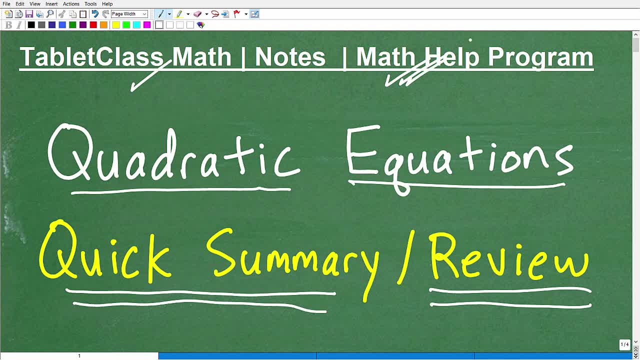 I also have tons of specialty courses, especially in the area of test preparation. So if you're studying for a test, you're going to want to go to Tablet Class Math And I'm going to give you tests like the GED, SAT, ACT, teacher certification exam, Accuplacer, Alex, There's a ton of different. 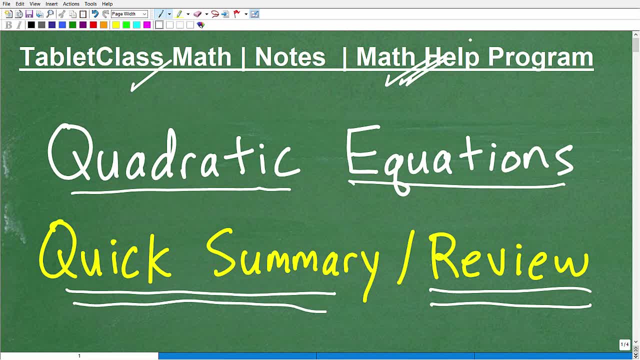 reasons why people study mathematics outside of a math class. So if you're studying for one of those tests, just go to my site, check out our course catalog. I should have your test of it. Don't drop me a line and I'll give you my best suggestion. I also work with independent 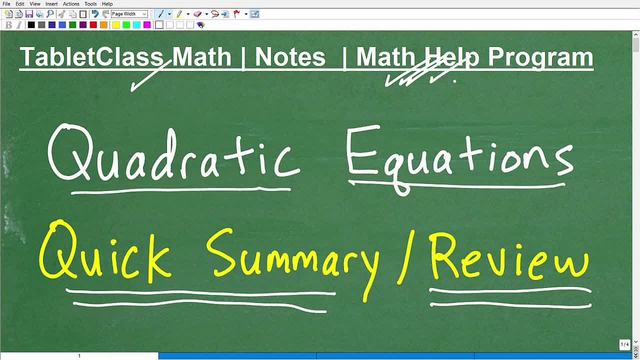 learners like homeschoolers. I have a great homeschool learning program And then obviously I help those of you out there just struggling in your math class. But one thing you can be doing to help yourself out in mathematics is to be taking great math notes. It's kind of my golden rule of math over decades of teaching it. Just one thing is. 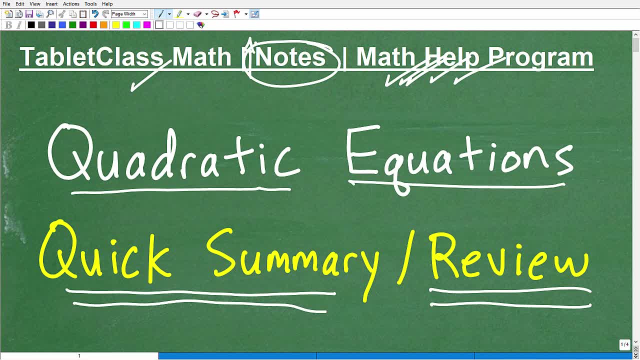 absolutely clear to me: Those students who take great math notes almost always end up with great math grades, And the reverse is true. Those students are, just like you know, like to look at their phone and talk to their friends. I get it, I was a young person once And, by the way, 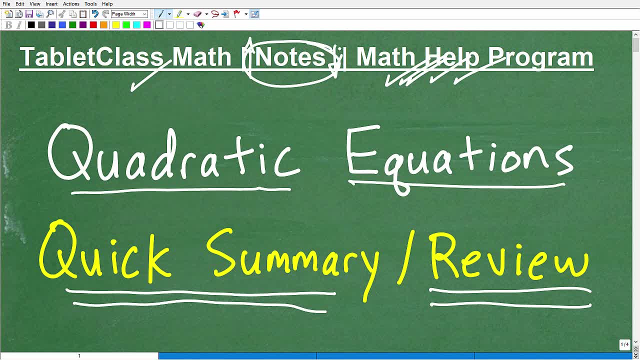 too. if I had a cell phone when I was, you know, a student, I don't even think I would pass. So we have a lot of distractions, And the only way to keep yourself not distracted is to engage in an activity that's going to keep you focused, And that is note taking. Okay, so improve on your. 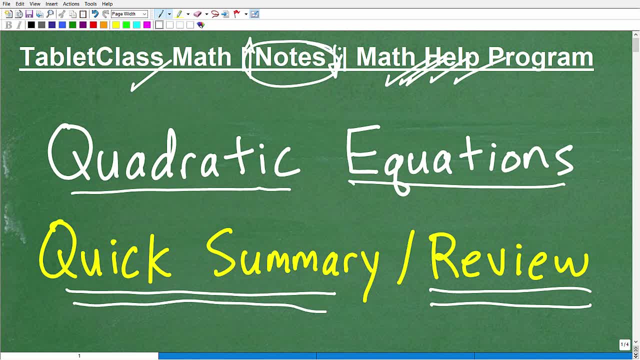 notes and your grade, Everything will get better. Okay, I promise you that Now. in the meantime, you need something to study from, So I actually offer detailed, comprehensive math notes to include pre-algebra, algebra one, geometry, algebra two and trigonometry. You can find links to those. 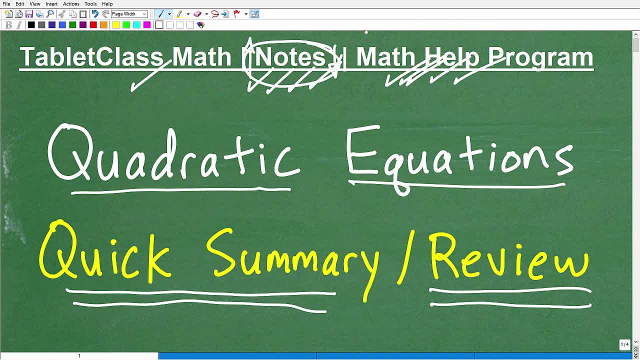 notes in the description of this video. So if you want some more detailed notes on quadratic equations, I would suggest, like my algebra one notes or algebra two notes. Okay, All right, And obviously if you really really want to master this stuff, I would suggest my algebra one or 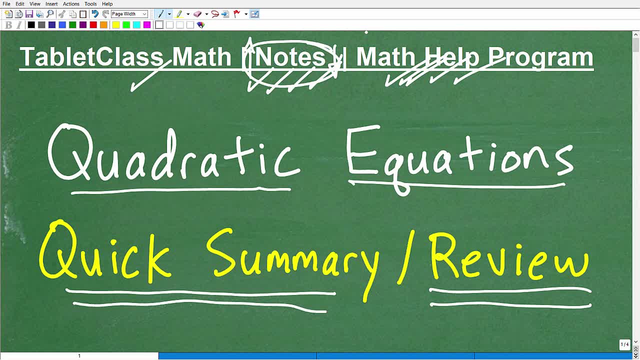 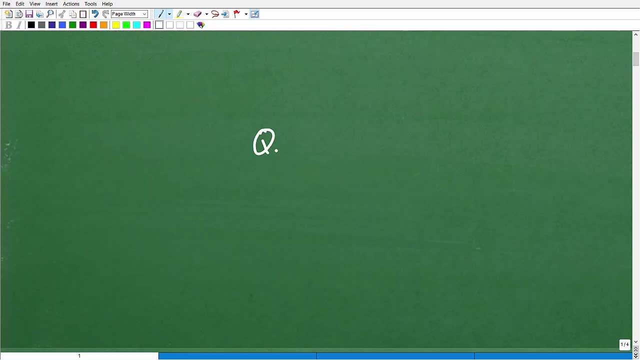 algebra two course, because you're going to really, you know, like get really deep into the stuff and master it. You'll end up with like an outstanding grade on your test, I'm sure. Okay, so let's get into quadratic equations. a quick summary of it And let's just put it down right here: Quadratic. 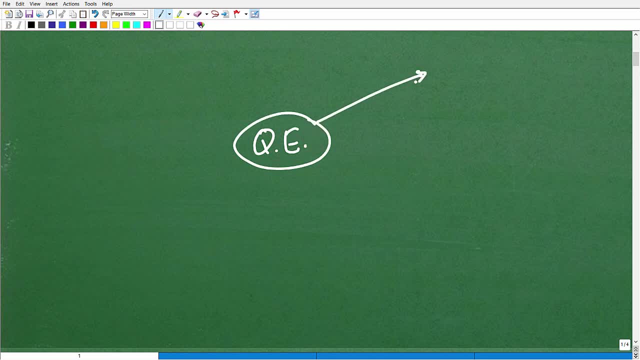 equations, And we'll get into it by starting off. What are quadratic equations? Okay, so this is the first thing you need to know: What is a quadratic equation? Well, it is a polynomial. All right, we need to know that quadratic equations are polynomials and they're degree two, degree two. 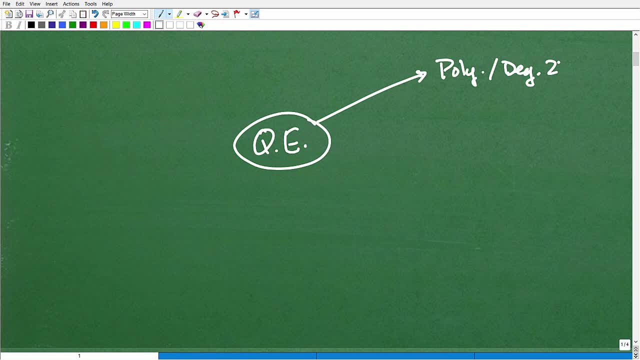 polynomials. That's what they are. Okay so, but what does that mean? Okay, well, it means that there's something called- and we'll just kind of put it in here in a little graphic kind of way To kind of summarize quadratic equations- There's something called the fundamental theorem of. 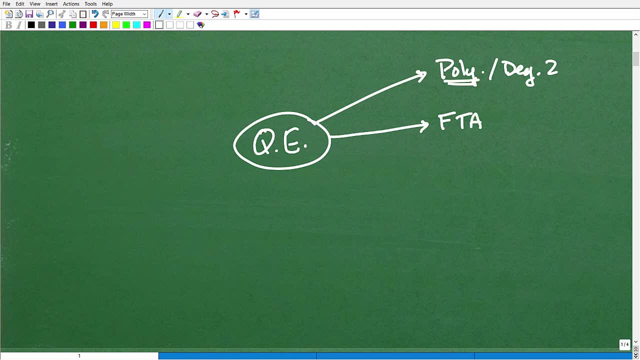 algebra that states that if you're dealing with a polynomial, okay, how many solutions that polynomial equation will have is going to be equal to the degree of that polynomial. So the fundamental theorem of algebra states that, oh, degree two polynomials are, by definition, 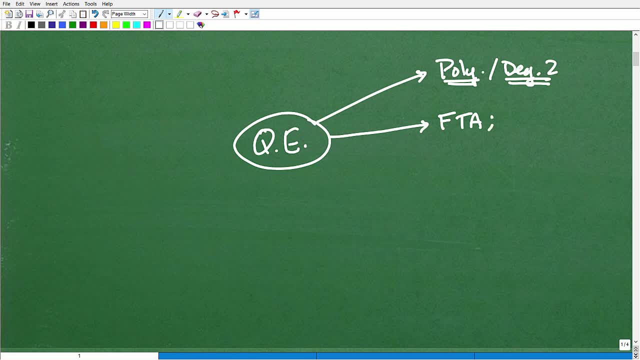 quadratic equations. So that means that all quadratic equations all will have a: two solutions, always Okay. so when you're solving quadratic equations, that's a big part. If you're studying quadratic equations or quadratic functions, a huge part of what you study is how to 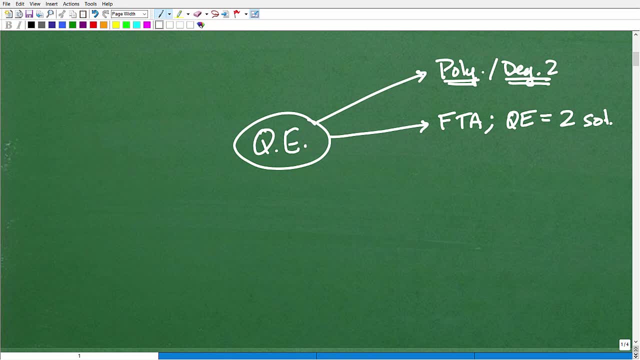 solve quadratic equations. Okay, just know this: that you will always have two solutions, Always, always, always. Why? Because a quadratic equation is a polynomial. Okay, it's a degree two polynomial And a fundamental theorem of algebra tells us that a quadratic equation is a polynomial. 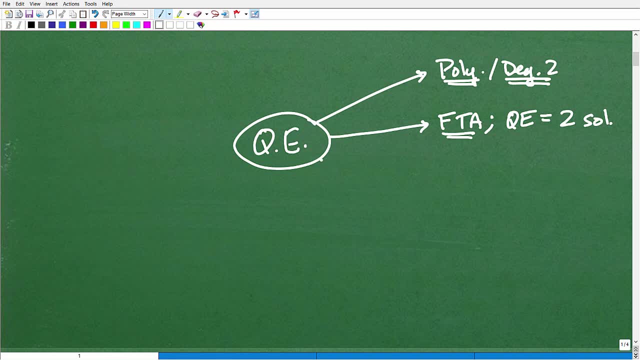 So that degree two, polynomials will always have two solutions. Now, what type of solutions do polynomials have? Okay, so two solutions, All right. So what type of solutions? Well, they're going to either be two real numbers, or you're going to have two imaginary or complex. 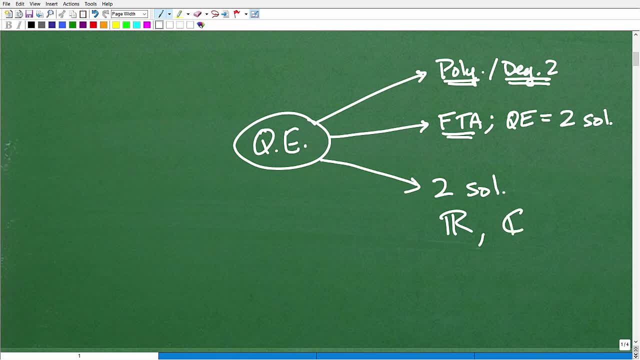 numbers. Okay, so you need to know something about imaginary numbers. So I'll give you a quick example over here. Let's take this basic quadratic equation: x squared is equal to 16.. All right, so this is a quadratic equation And we're going to have two real numbers And we're 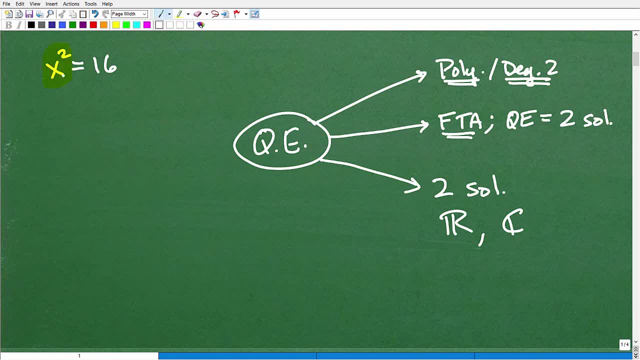 going to have two imaginary numbers. So this is a polynomial. Okay, it's a degree two polynomial. Now, this is the easiest quadratic equation you'll ever have on a test. I'm pretty sure your teacher may not even put this in and be like that's too easy. But I don't know, maybe you have a nice. 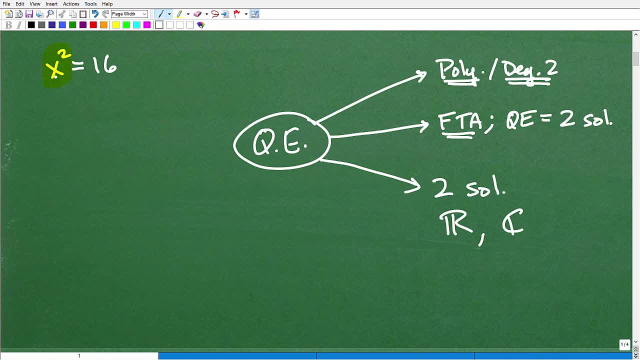 easy teacher, And that's awesome if you do, But let's go ahead and just solve this right. So how do we solve that? Well, we have to take the square root of both sides, So x is going to be equal to. 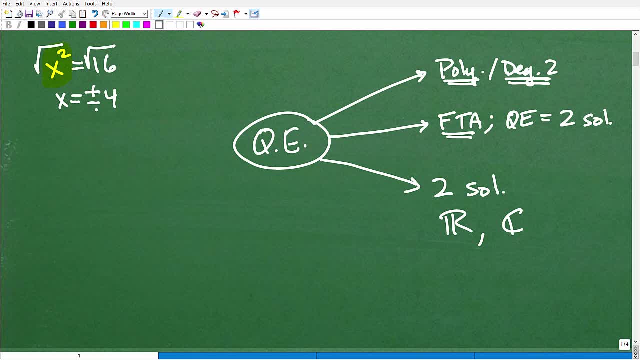 positive and negative four. the square root of a positive 16 is positive and negative four. All means that x is equal to four. that's one solution, And our second solution is negative four. So those are our two solutions to this real, basic quadratic equation. Now, how about this quadratic equation? 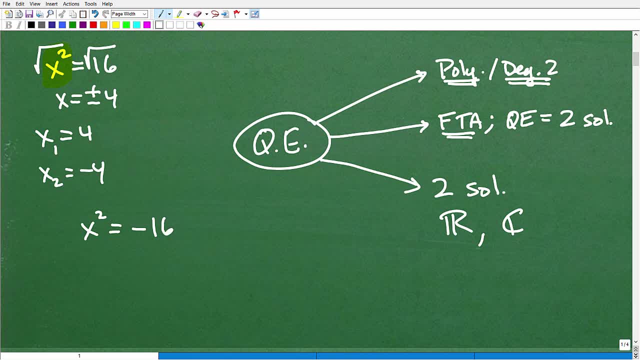 x squared is equal to negative 16.. All right, well, you need to know how to deal with these guys. If you try to take the square root of both sides- and you should, okay- and if you're going to your calculator and take the square root of negative 16, you are going to have an expression like this: 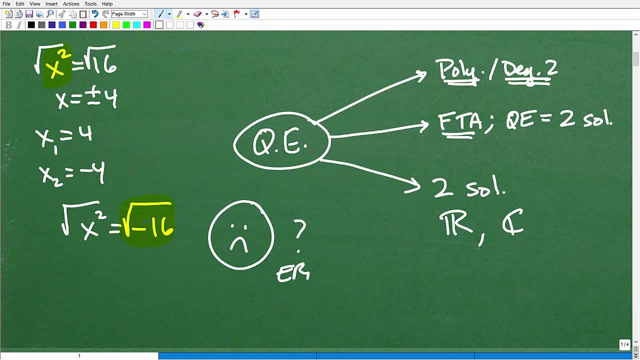 You're going to be like: I don't understand what my calculator is telling me. It's giving me some sort of error because your calculator is kind of set to deal with real numbers. Now you can interpret and set up your graphic calculator and scientific calculator to work in imaginary numbers. 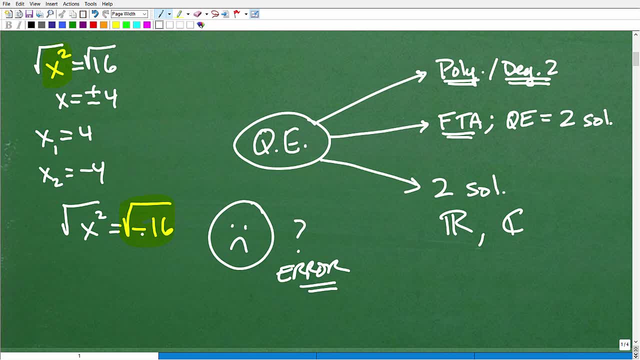 But you've got to know something about imaginary complex numbers just to be able to interpret your calculator. So in this situation, let's just kind of go back here, take a step Back. we have x squared is equal to negative 16.. 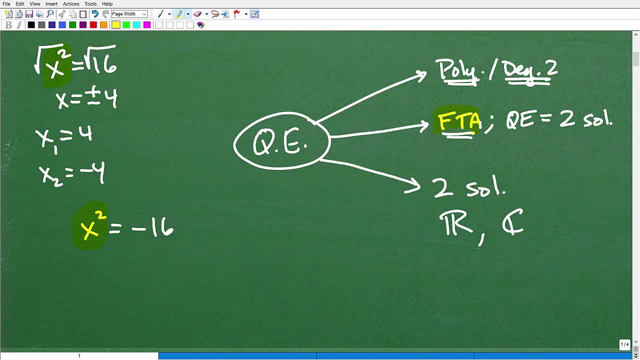 Well, this is a quadratic equation And the fundamental theorem of algebra tells me there is two solutions. So there are solutions to this. It's not like I can't do this, My calculator doesn't like that. No, there are two solutions. 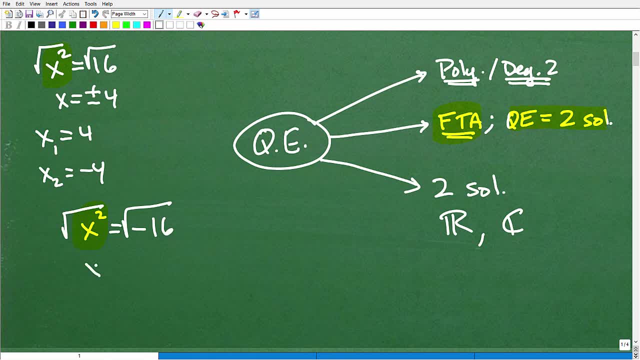 And the way I go about it is to take the square root of both sides. But x is going to be equal to positive and negative. for i Now this video. I cannot possibly teach you all these subsets of things We're doing it. 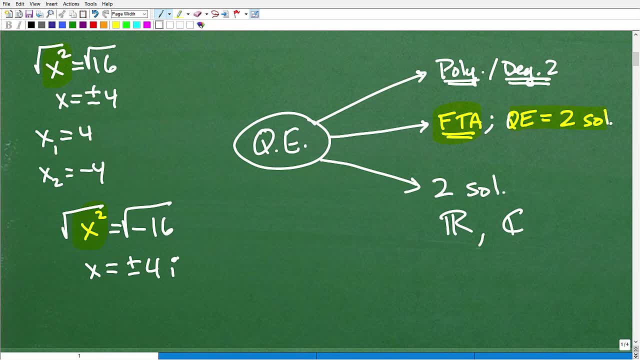 It's a quick review Now. a couple of suggestions here. All right, If you're struggling with quadratic equations, I have tons of videos on quadratic equations and all these kind of subtopics within my algebra and algebra to playlist on my YouTube channel. 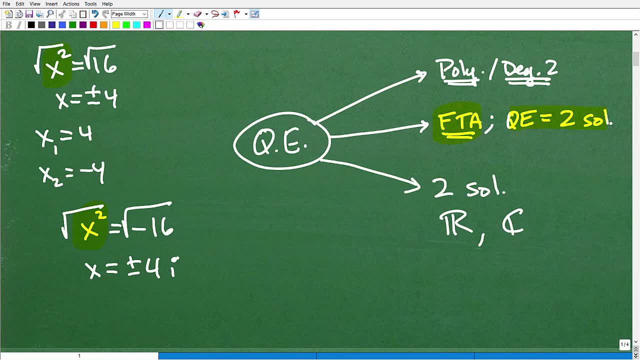 But if you really want to know this, I would say you can jump into maybe my algebra one or algebra to course in my math program And you know you're going to see a ton of instruction and example. problems are really, really helping prepare for any particular exam that you might be taking. 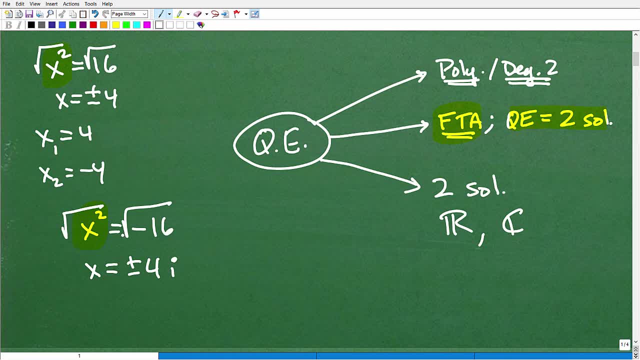 All right. So just so you know, I'm just trying to make the point here. There's always two solutions, either real number or imaginary complex. OK, All right, So let's erase this and continue on with our discussion of quadratic equations, everyone's favorite topic. 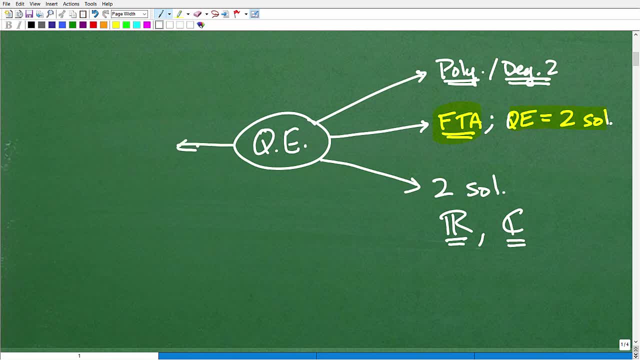 So let's start over here. How do we solve quadratic equations? OK, Well, there's a number of different ways we can solve quadratic equations- Not a crazy number. There are different ways, but it all depends on the situation. We can take the square root of both sides. 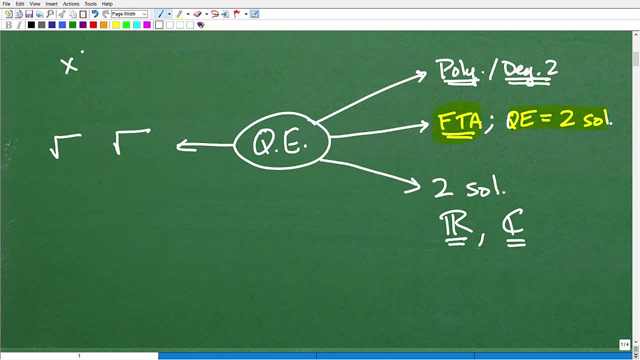 OK, We want to try to take the square root of both sides, if we can. That would be an example like this guy right here: X squared is equal to 16.. If I take the square root of both sides, OK, I can solve this type of quadratic equation where there's no X term, like so: 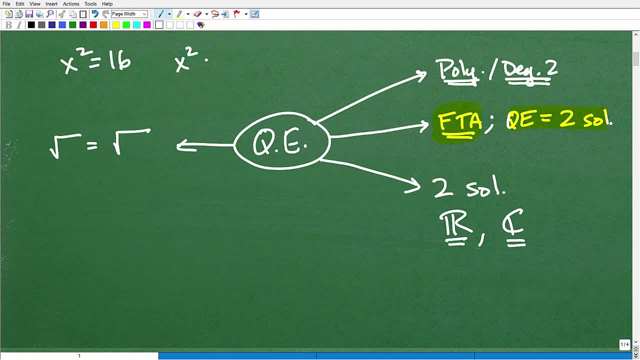 That works out OK, But what happens if I have X squared plus X equals 16?? Well, now I cannot. I take the square root of both sides, So I need other techniques, OK, And those other techniques would include factoring. 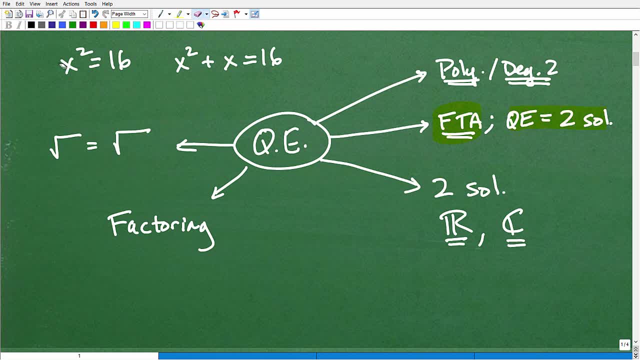 All right, So factoring is an excellent technique to solve quadratic equations. So when you factor, let's kind of look at something like this: X squared plus X equals zero. OK, So this is a basic quadratic equation. All right, So we have a polynomial degree two. 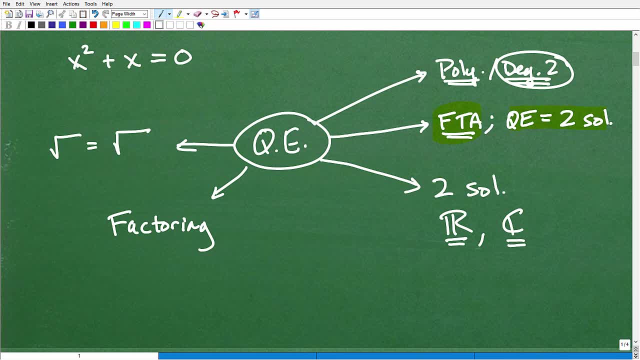 And by the degree the degree of a polynomial is, it's the highest power. OK, So this is a degree two. This is a first degree term. This is to the first power, But this highest power of this polynomial is two. So that means that it's a degree two polynomial. 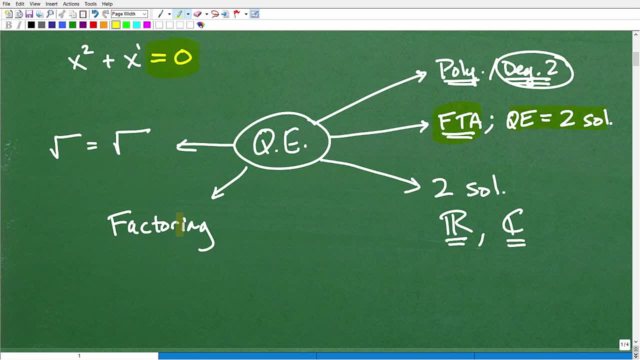 But to solve this, if we have this thing set equal to zero and we can factor- you want a factor? OK, I would not take the square root of both sides by moving this, This term, over the to the other side like this. that's not going to help us out. 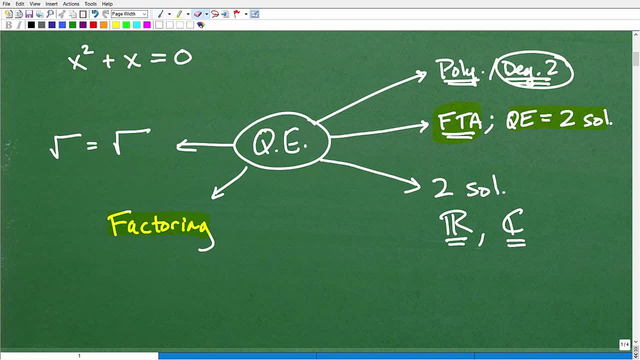 So you need to be able to recognize patterns in terms of factoring. So if I can factor this, which I can, and it's set equal to zero, OK, This right here. you have to have this thing set equal to zero. 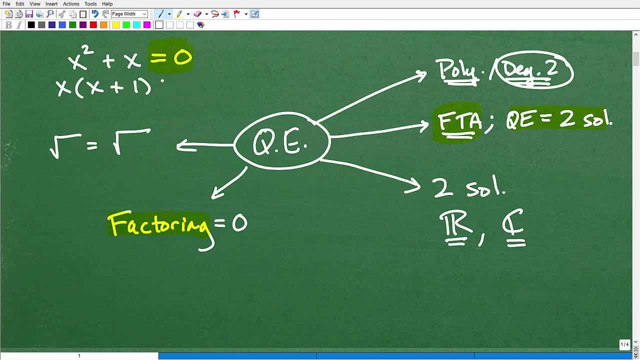 So this would be: X times X plus one is equal to zero. All right, Now this case: if you can factor, you should definitely factor again. The equation has to be set equal to zero, And then you set Each factor equal to zero. 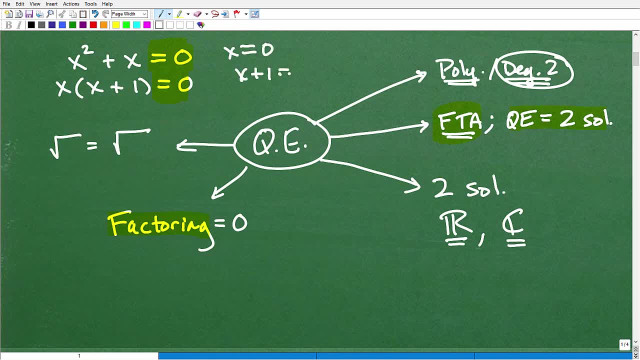 So in this case, X is equal to zero and X plus one is equal to zero. So this is one solution And X equals negative. one is the other solution. So this is a great technique to do, OK. So factoring, if the situation calls for it, the square root of both sides, if the situation calls for it, if you can. 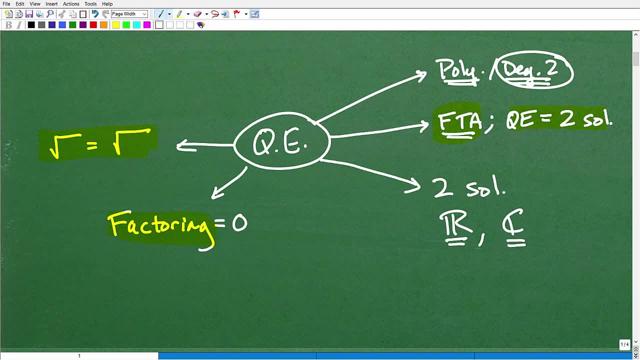 OK now factoring, by the way, will require you to know how to factor the greatest common factor And oftentimes trinomials. So if you can't factor trinomials or greatest common factor or other type of factoring situations, you're going to really struggle with quadratic equations. 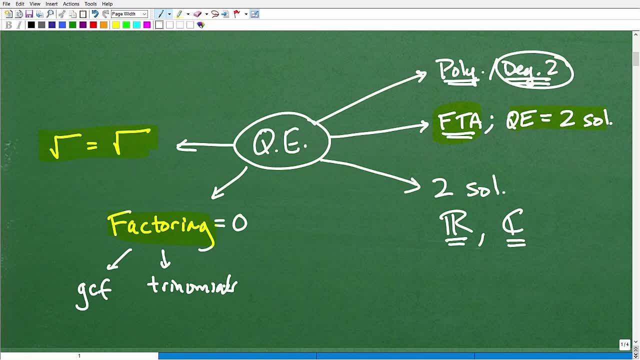 You need to boost your factoring skills. OK, Again, you know all these sub skills. if you need help on them, check out my other videos in my algebra channel. I'm sorry, as a playlist on my YouTube channel, or just you know, jump into my algebra course. 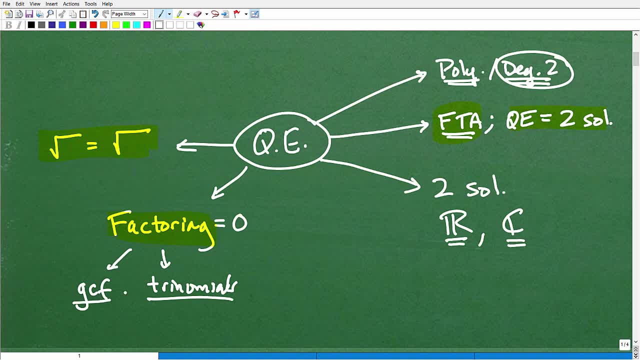 But again, you need to know how to factor trinomials, greatest common factors, Because This will be a situation that your, your teacher will expect you to be able to solve. Now, what happens if you can't take the square root of both sides and you can't factor? 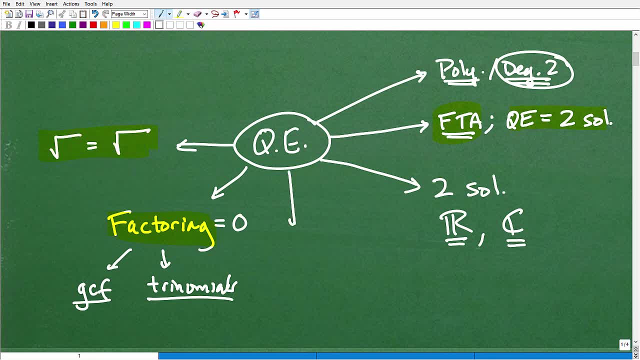 OK, what about in that situation? Well, we have something called the quadratic formula And we love the quadratic formula. It is awesome Here. it is right here. You need to know this thing by heart. X equals minus B plus minus square root of B squared minus 4AC. 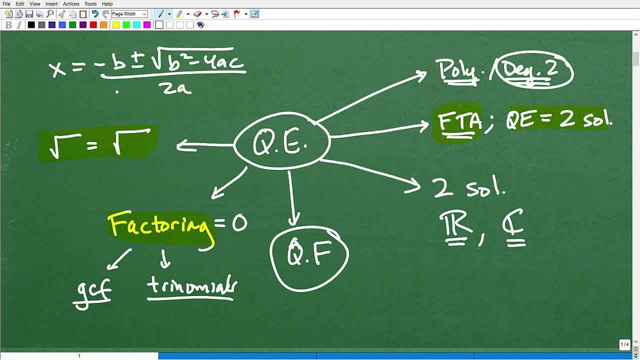 All over 2A. So if we're talking about the coefficients of a polynomial, AX squared plus BX plus C is equal to zero. This should be familiar to you. OK, if you're taking a quadratic equations test, you need to know how to work with the quadratic formula. 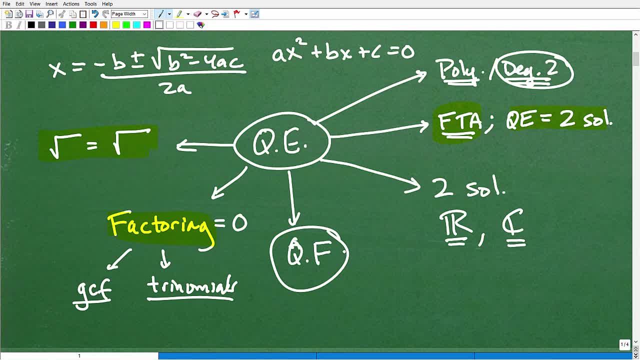 Again, I have tons of videos on this. but basically the quadratic formula is our technique of last resort. If I can't take the square root of both sides, if I can't factor Well, then I have to then default to the quadratic formula. 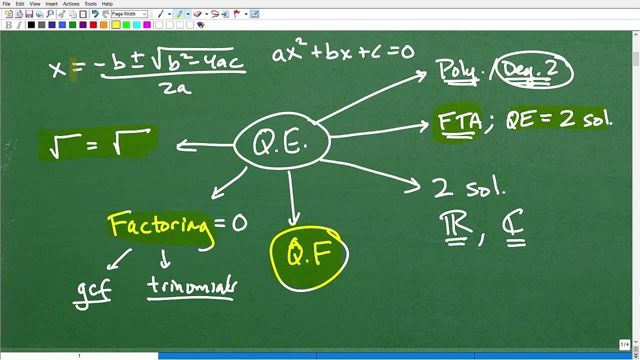 You don't want to pick the quadratic formula as your first, primary way of solving a quadratic equation. You don't want to do that. OK, you want to see if you can use these other techniques And if you can't. if something can't be factored, you can't do this. 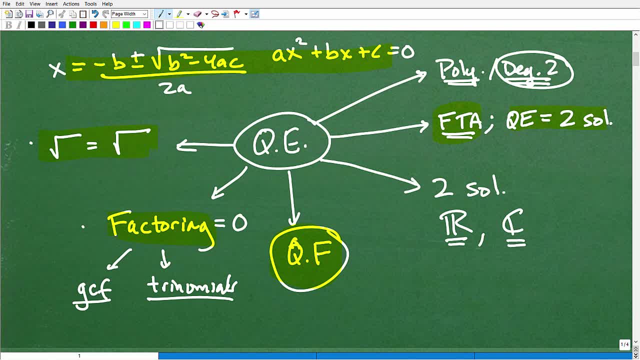 Well then, then you just jump into the quadratic formula. Remember, there's always going to be two solutions, because there's always going to be a way to find these solutions. So if you can't factor, you can't take the square root of both sides, then we have to. 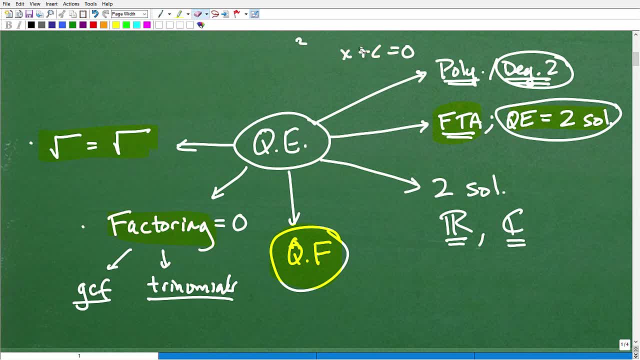 Use the quadratic formula. So knowing how to use a quadratic formula and avoid common mistakes is critical. OK, so you need to understand that for sure. Now a long way of doing the quadratic formula. The quadratic formula is actually a shortcut of something called completing the square. 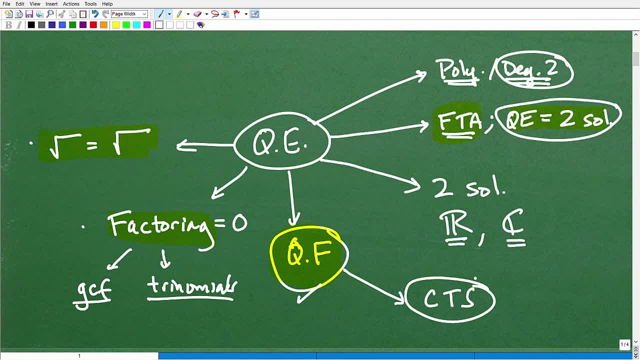 You need to know how to use, how to do the complete the square. OK, but completing the square is not a primary technique technique. You can actually solve Quadratic equations by completing the square and you will be asked to do this on test. 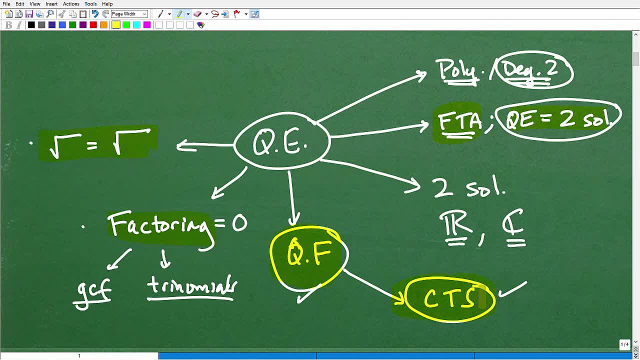 But I want you to realize that in a practical sense completing the square is a long version of the quadratic formula And there's a whole discussion behind that. But just kind of trust me on this one You don't use. completing the square is kind of like a primary technique. 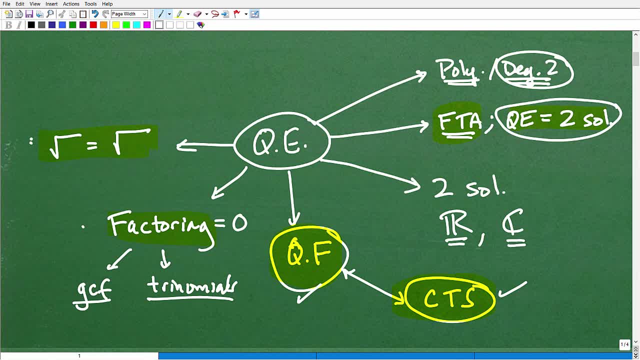 OK, if you can't solve a quadratic equation by these techniques here, then you're going to use a quadratic formula. You would just start using and complete the square, And I'm kind of speaking in generalities, but that's a good way to kind of think of it. 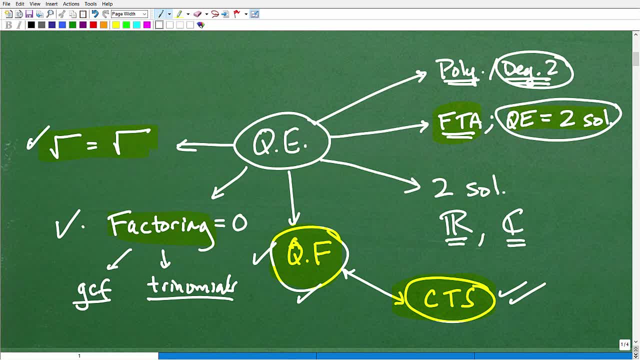 But you need, you definitely need, to know how to complete the square, And this confuses a lot of students, Right? So you can see, on a quadratic equations test, there is, you know, a lot involved. OK, now let's get back to the type of solutions a quadratic equation has. 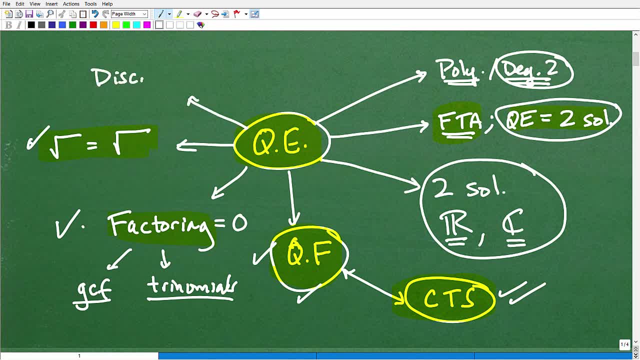 So there you're going to need to know something called the discriminant. OK, the discriminant. Let me go ahead and put that quadratic Formula back up: B squared minus four, AC all over to a. this part right here of the quadratic formula is called the discriminant. 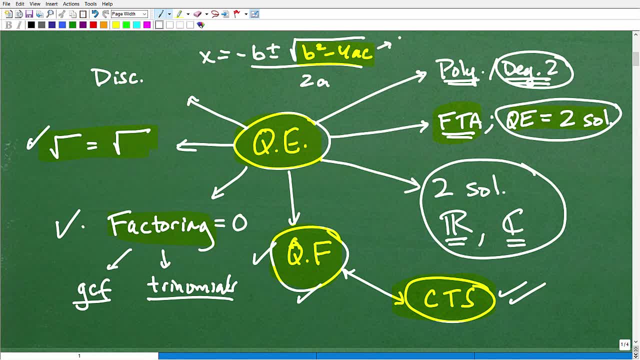 You need to understand that And this, depending on whether it's a positive value, a negative value or zero, will determine. Well, basically, as an indicator to tell us what type of solutions and roots we're going to have in our quadratic equation. 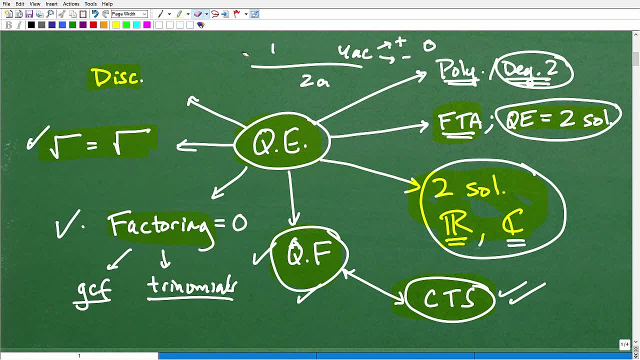 So you need to know about the discriminant again. You know I can't possibly teach all this in this video. There's just too much information. But check out my additional videos on my channel or again check out my algebra course. All right, So the discriminant- All right. 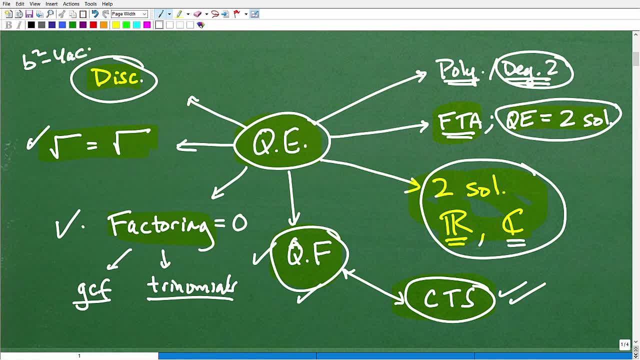 So that's the B squared minus four AC part of the quadratic formula. Now, along with all of this, some additional things you're going to need to know about quadratic equations is how to graph them. All right, And there's. this is a whole. 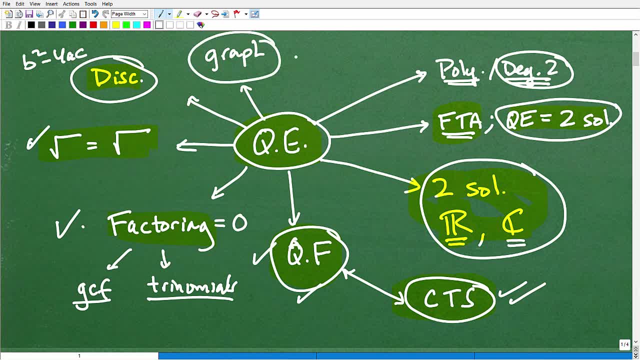 Other topic: how to graph quadratic equations. So we're talking about parabolas, OK, and you need to know where the vertex is, that you need to know the axis of symmetry. There's a lot of stuff about just how to graph. you know parabolas. 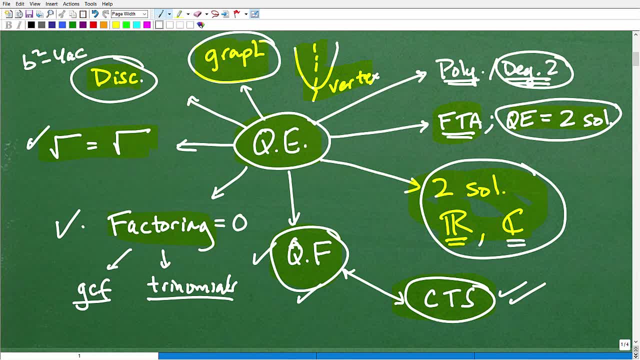 Again. I have additional videos on that, but you're going to need to know this. OK, how to find the vertex whether the parabola is this way or this way, if it's wide skinny- all that kind of good stuff. 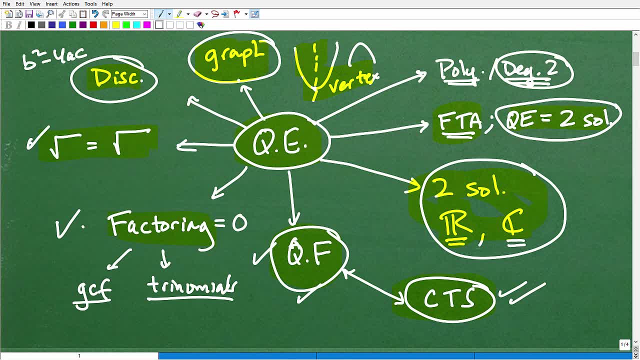 And then one last thing That you often see On a quadratic equation Test is quadratic inequality. So let's kind of squeeze this guy over here- Inequalities, I'll just kind of abbreviate like so. So instead of a quadratic equation you'll actually have an inequality symbol, and that is a whole nother set of techniques that you're going to have to follow. 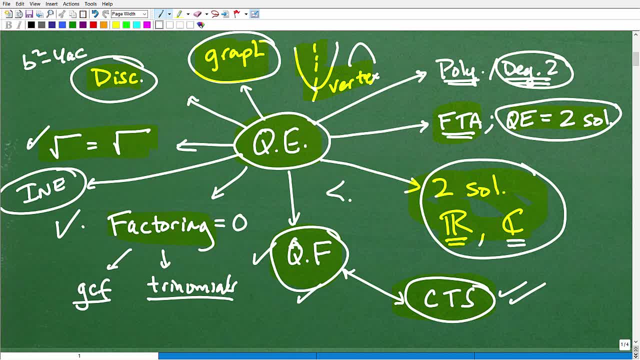 So there is a huge amount of information in a quadratic equations test. This is kind of a structure summary of what you're going to Be be facing. all right, and you don't want to be weak at any of these particular areas. so even about 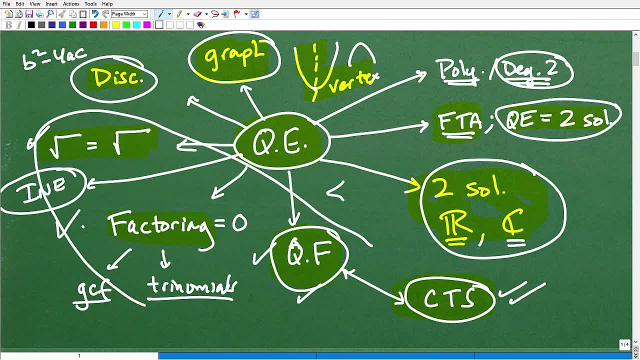 like how to solve quadratic equations. you need to know all of this stuff. okay, just to even handle quadratic equations, but there's going to be test questions. um on, hey, you know, graph the quadratic equation. uh, use completing the square. what type of roots or solutions does this quadratic? 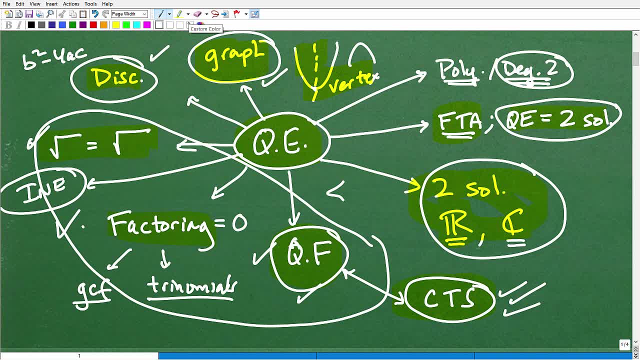 equation have your teachers want to want to see your understanding the discriminant, which means you need to understand how to deal with imaginary numbers, real numbers. you know it's all. it's a lot. okay. now, if you're some, you're taking a real basic. you know algebra course and your teachers 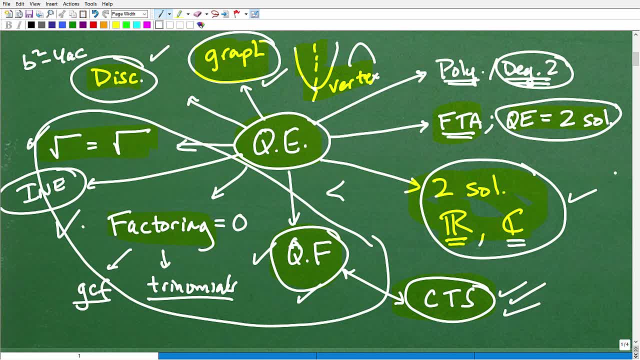 give you some basic questions. well then, that's fine too, but just so you know, you're really not mastering this huge, very, very important topic in algebra if you don't know all these uh things right here. okay, so don't, don't panic. and by the way too, we haven't even talked about word problems. okay, so quadratic. 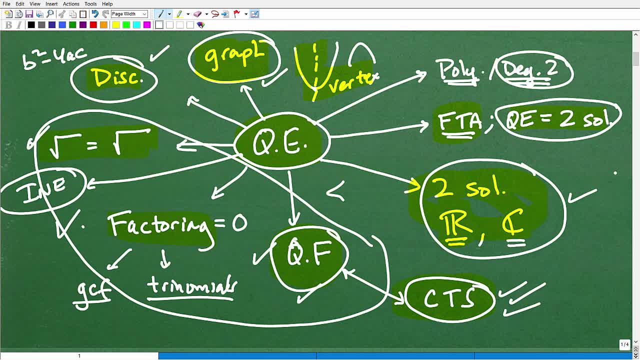 equation, word problems. so mathematics it's, it's a lot, okay, uh, this you know. the whole purpose of this video is to help organize what you need to know for this test. so how do you get ready? well, okay, first of all you take a deep breath, you settle yourself down, but then you jump into 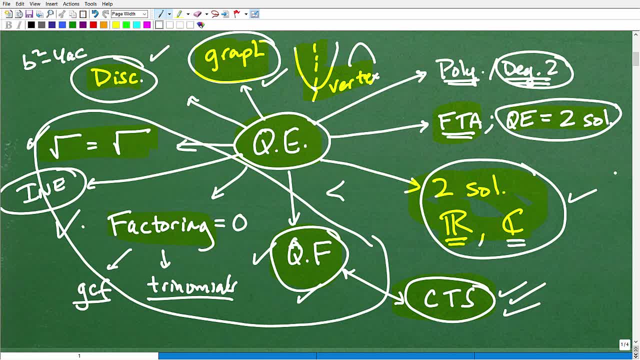 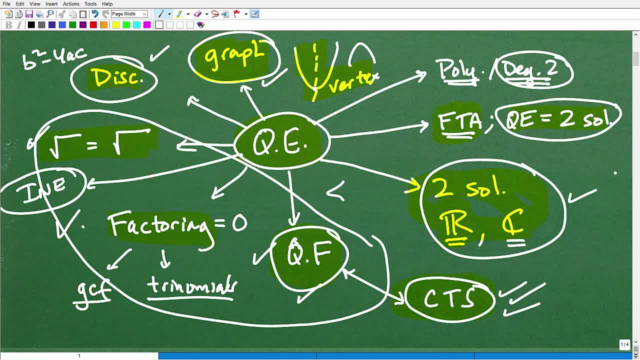 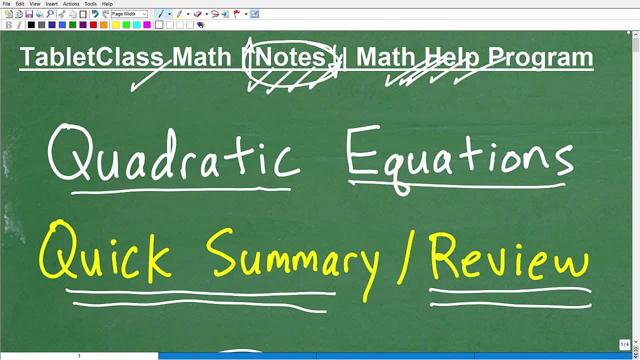 need something else so you can use my videos on my youtube channel or, in a more formal way, check out my course. but if you're going to be facing a quadratic equations test, okay, and you definitely will. if you're taking algebra or any course beyond that, this is the kind of stuff you 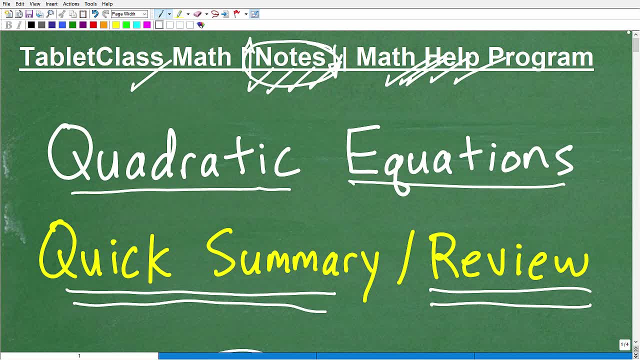 need to know right, and hopefully this video helped you organize your. you know test studying, you know strategy. okay, you got to hit all those different topics, all right. so if you found this video helpful, okay, please consider the smashing that like button and help me out. and, by the way, too, 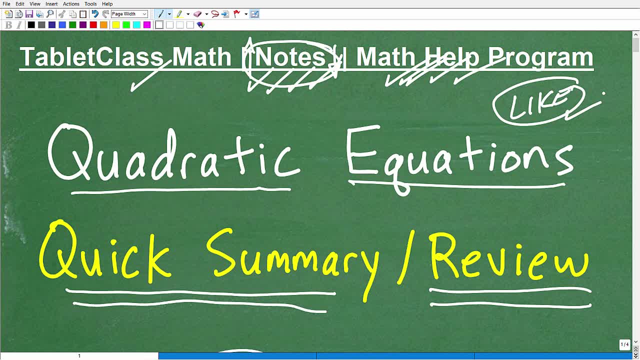 if i get a good response on this particular video, i think i'll do additional test summary videos and other major topics chapter test topics in in algebra and geometry, algebra 2 and the like. i think this video is definitely helpful because your teacher is going to do a quick. 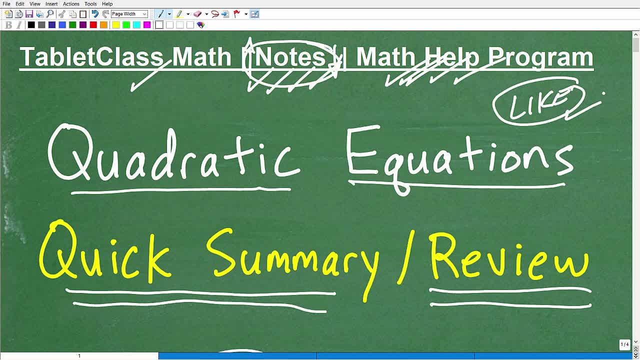 test review. generally, most teachers the day before um or day or two before we'll do a review like this- i know i did in my class and then that just helps, you know. summarize the main points. okay, i'm not reteaching everything because it's just too much information, but a summary of the main points will definitely.